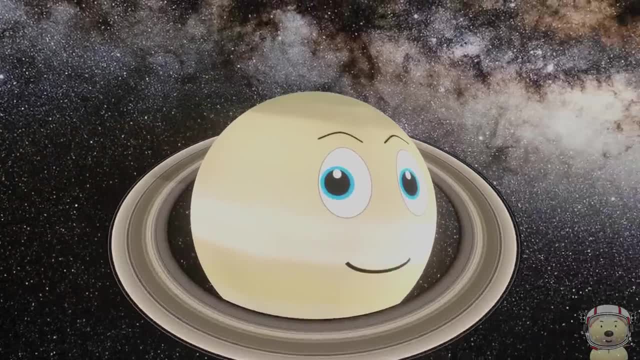 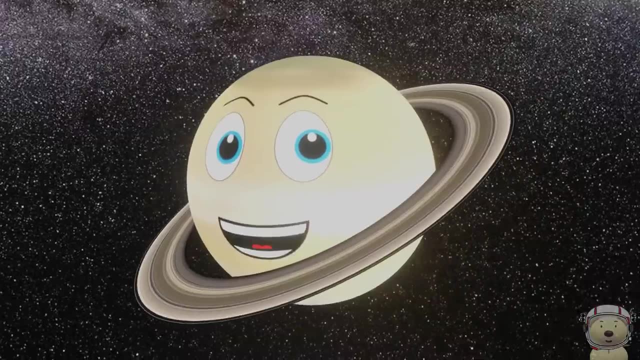 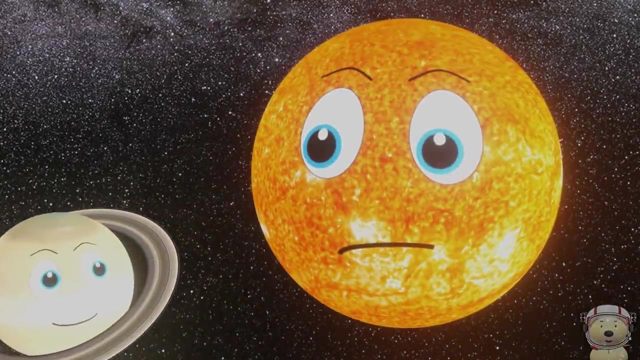 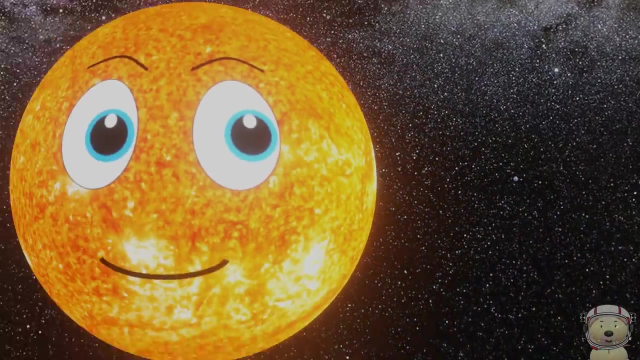 Hey everyone, my name is Saturn. Do you want to impress your friends with some amazing space facts? Well, keep watching. Our sun is a small dart, What? No way. Look how big I am compared to your Earth. I can fit 1.3 million of your Earth inside me. I think you're wrong, Saturn. 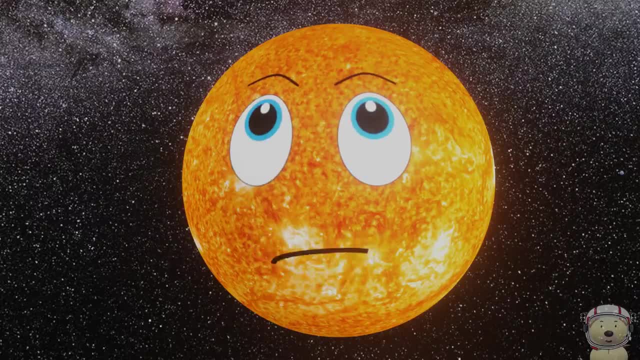 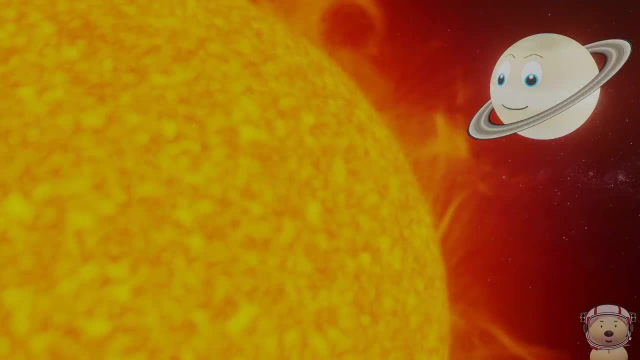 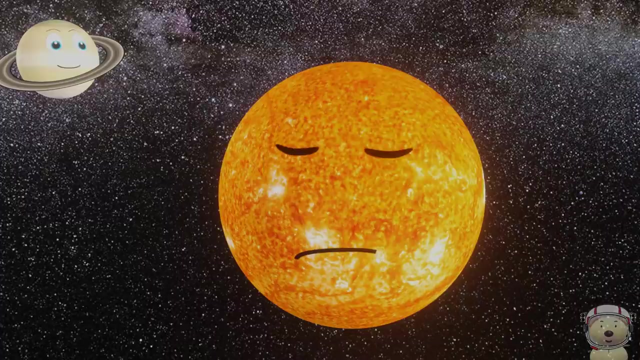 Hmm, Yes, but Apologise, please. But hang on, Apologise, please. No, hold on, Hear me out. You are a small dot compared to the largest known star in the universe. Oh, but I'm massive. I'm about 1.3 million kilometres in diameter. 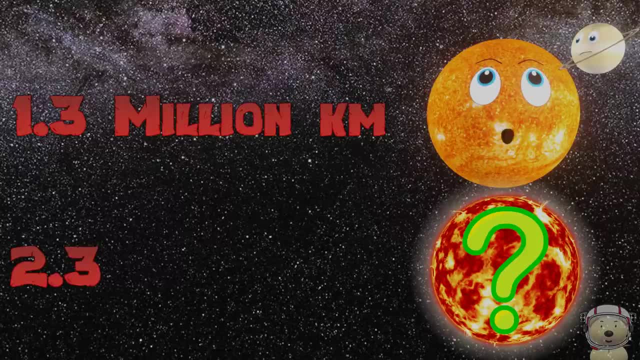 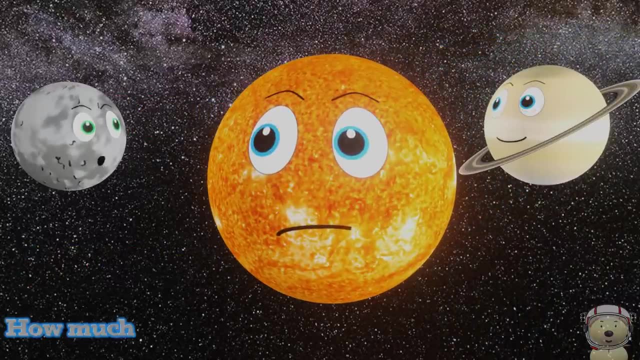 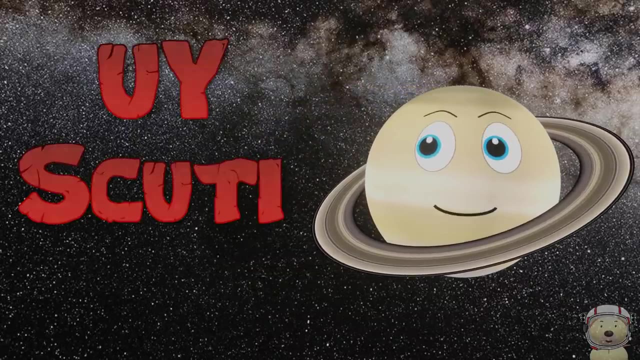 Well, this star is about 2.3.. Well, that's not much bigger. Billion kilometres, How much bigger is that than our sun? Well, this star, which is called UY Scuti, it has a radius that is 1,700 times bigger than our sun. 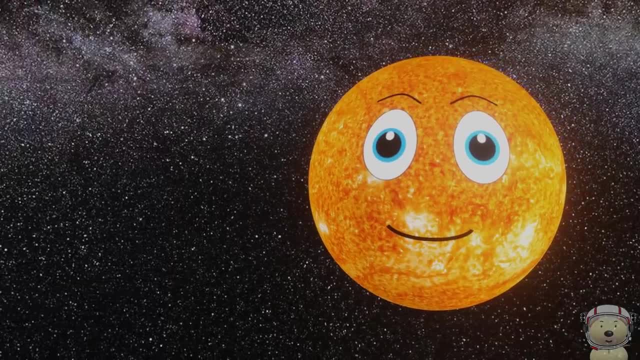 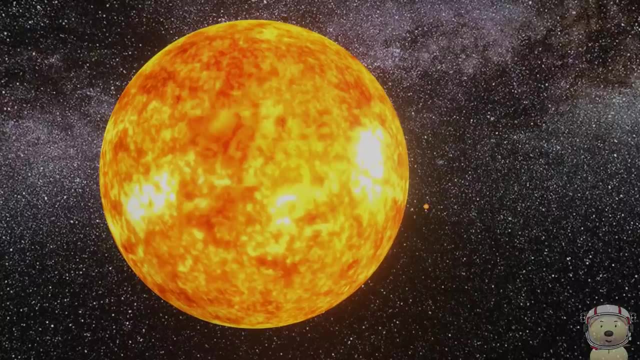 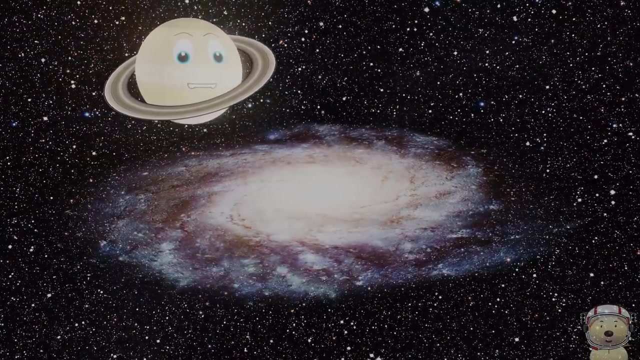 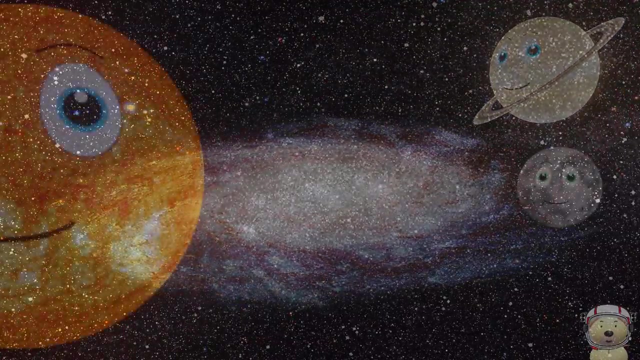 Oh my, Let's see what our sun would look like compared to UY Scuti. Uh, I'm tiny. UY Scuti is found in the middle of our galaxy, the Milky Way. Perhaps most amazing of all, if you replaced our sun with UY Scuti, its surface would stretch past. 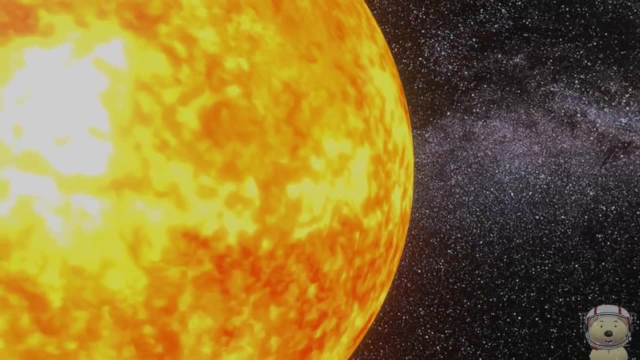 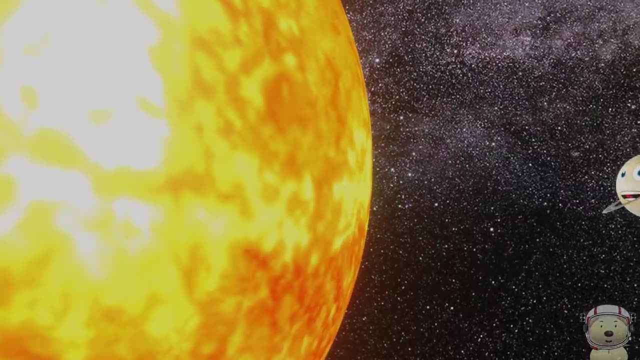 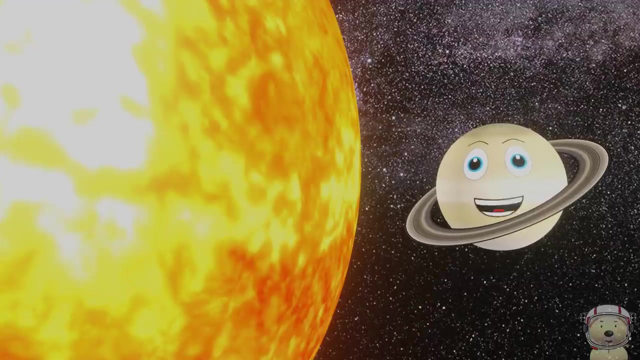 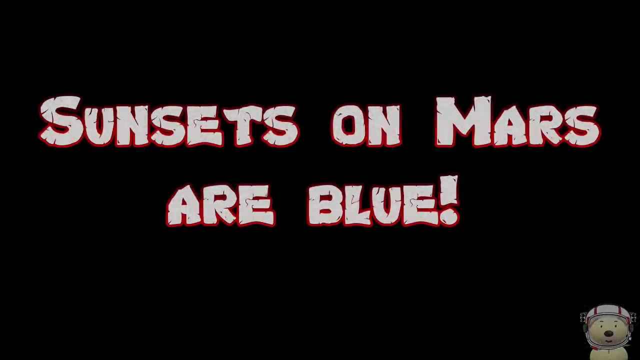 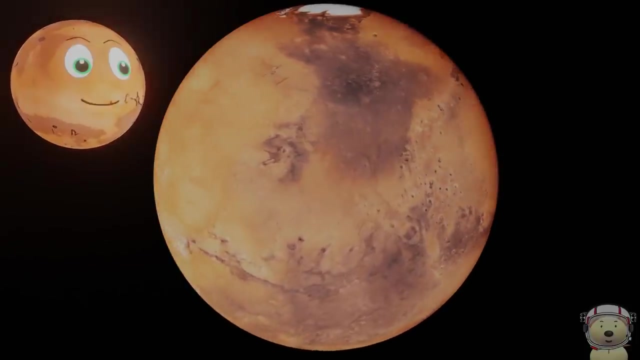 Mercury, Venus, Earth, Earth, Mars And beyond, Jupiter. That's massive, And there are probably bigger stars in the universe than that. We just haven't found them yet. Sunsets on Mars are blue. Hey, I'm Mars And sunsets on me, the red planet, are well. 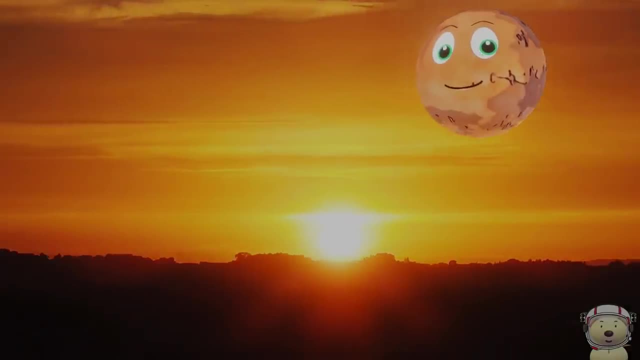 Sunsets on Mars are blue And sunsets on me, the red planet, are. well, Sunsets on Mars are green and south-south. Well, these are green day, aren't they? Oh, that's quite true. Well, these are well. 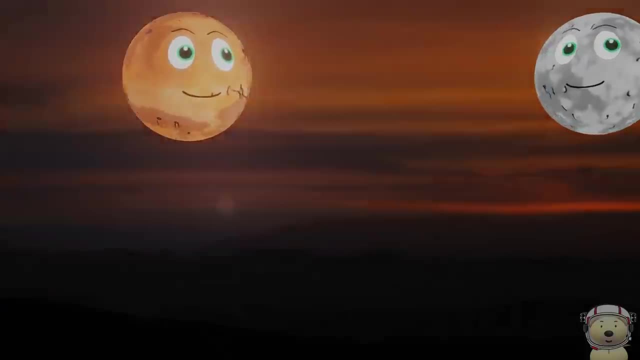 Blue On Earth. sunsets look yellow, orange and red. Well, are you sure they are blue? Yes, Take a look at this photo taken from the surface of me by NASA's Curiosity rover. Take a look at this photo taken from the surface of me by NASA's Curiosity rover. 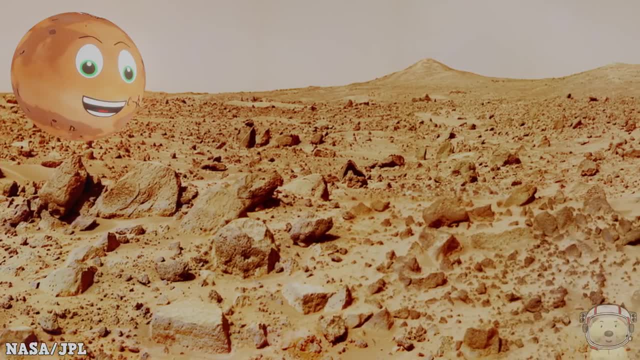 My atmosphere has fine dust in it, And this fine dust scatters red light so that the sky appears reddish, Which lets blue light through near the sun, And this fine dust scatters red light so that the sky appears reddish. 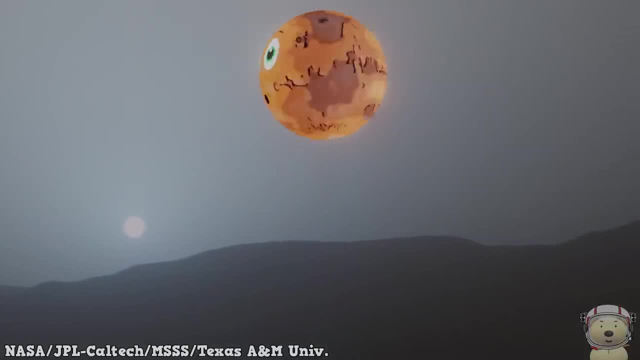 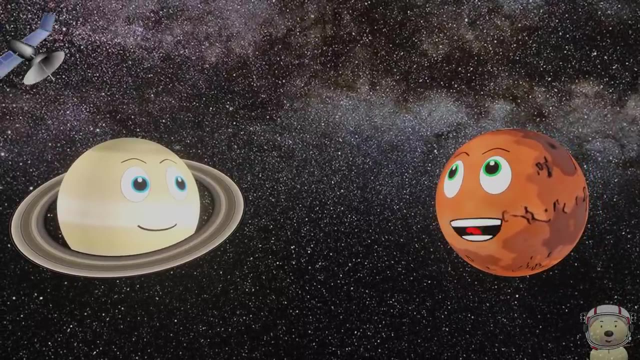 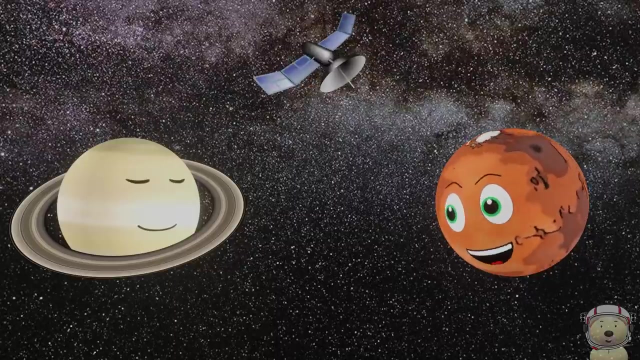 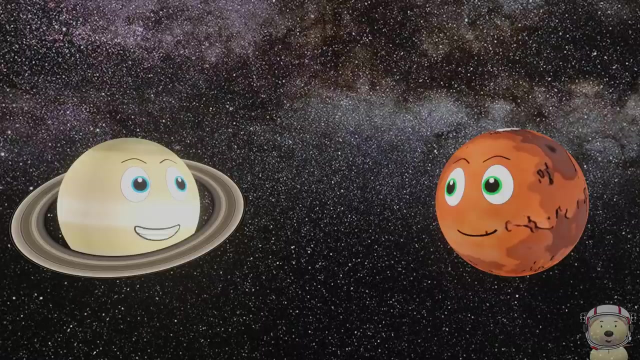 the sunset on earth. it's the other way around. that looks really cool. that's not cool. I'll show you cool satellite, give me a beat. my name is Mars and my sunsets are so cool. okay, okay, Mars, I believe you. let's hear the rest of the song later. 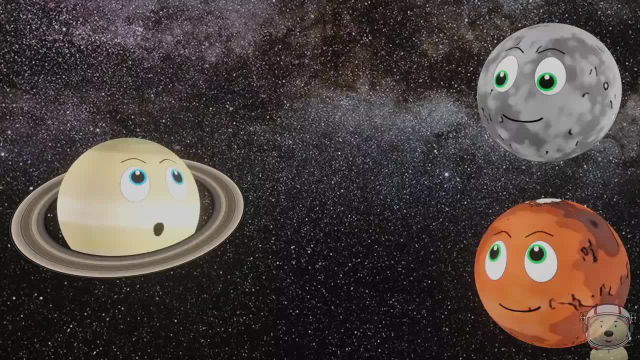 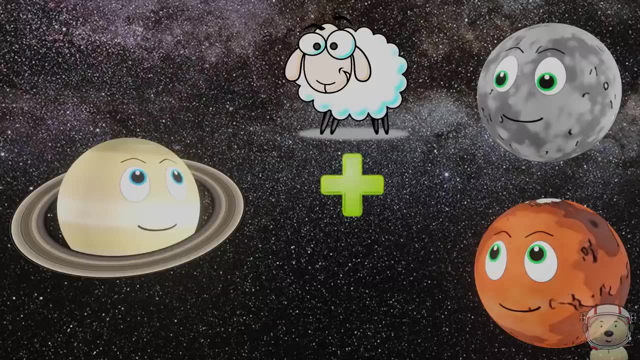 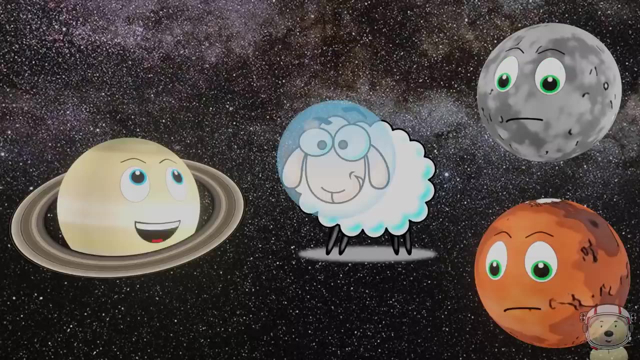 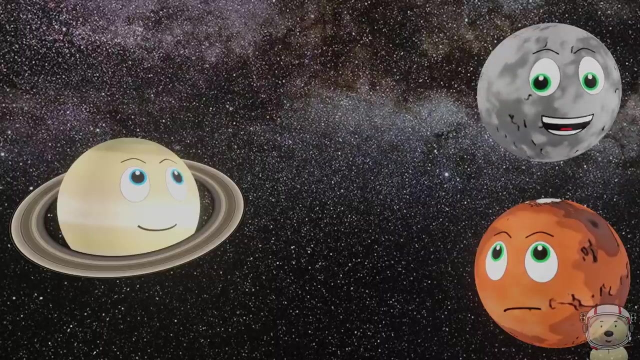 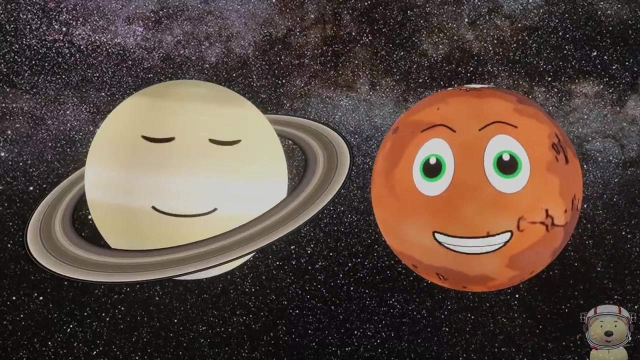 hey, Mercury, I've got a space joke for you. oh great, another joke. what do you get when you cross a lamb and a rocket? I don't know? a spaceship, spaceship, spaceship. get it. I don't even get paid for this. hmm well, anyway, you next time your friends or family want an awesome space fact, tell them: sunsets on. 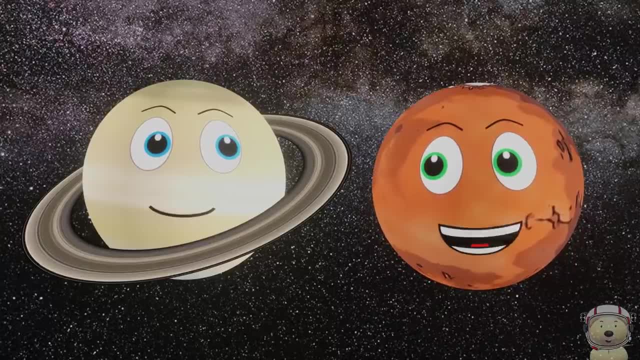 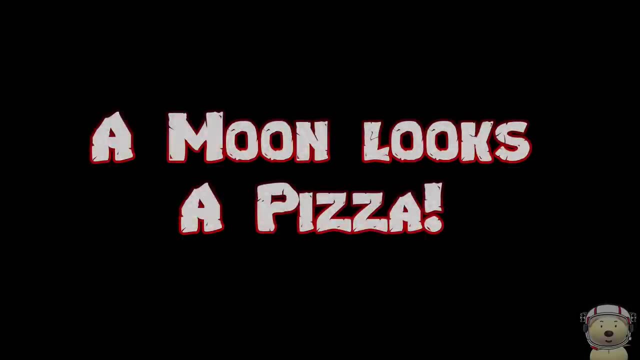 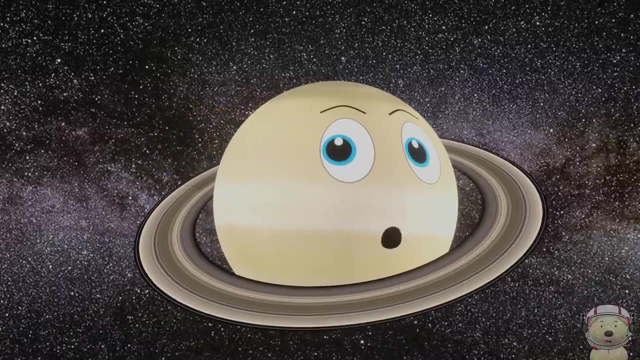 Mars are blue. that sheep joke was rubbish, I know. quick fact: a moon looks like a pizza. there is a moon in our solar system that looks like a pizza. do you know which moon it is? if you didn't know, the moon that looks like a pizza is: 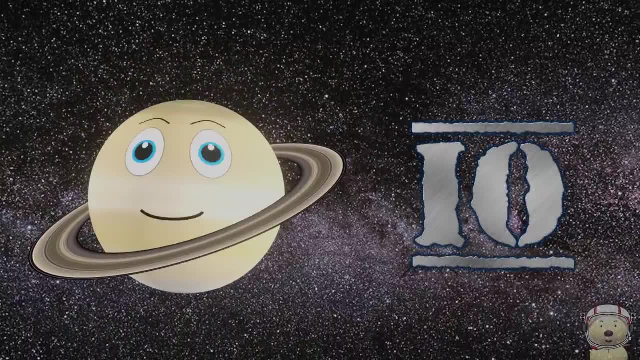 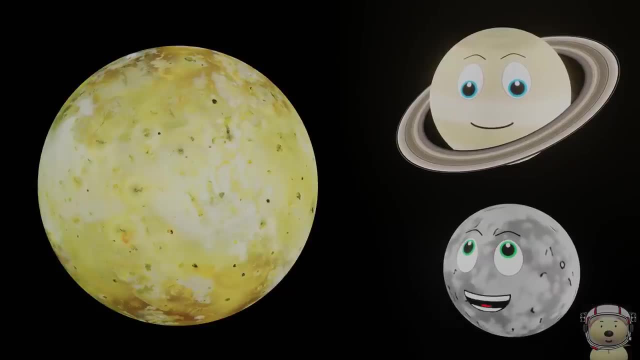 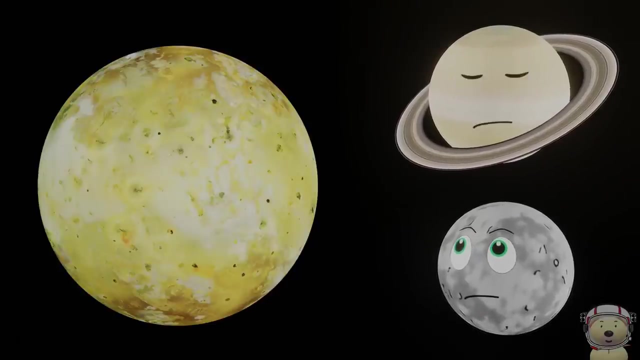 Io, Io, a moon of Jupiter. it looks like this because it is covered in volcanic craters. nice pizza, can I have a slice? no, no, it's a moon, not a pizza. come on, don't kick the pizza all to yourself. no, it's a moon, honestly, sure. come on, just a small. 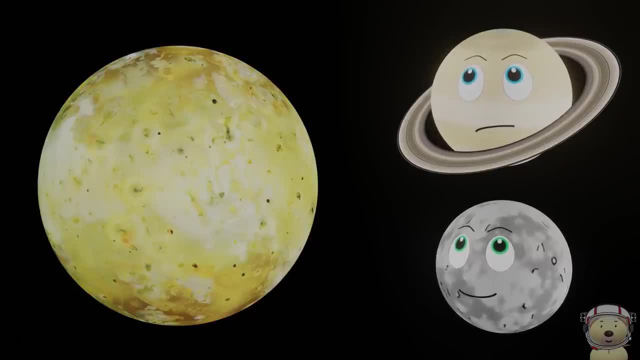 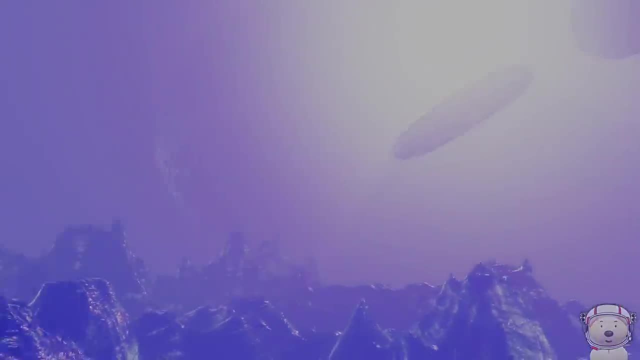 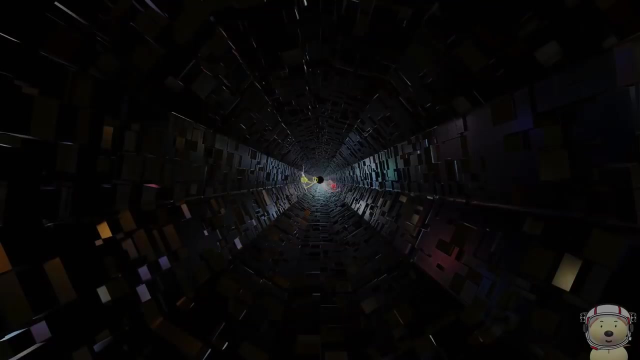 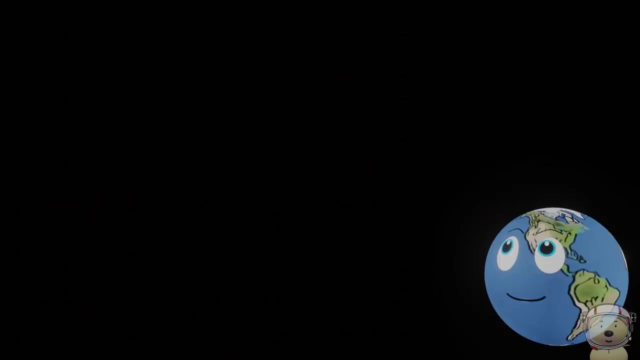 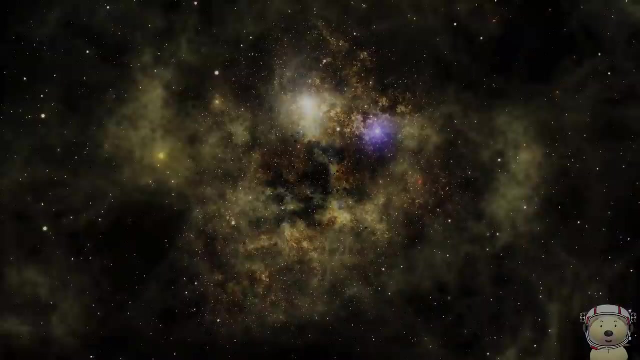 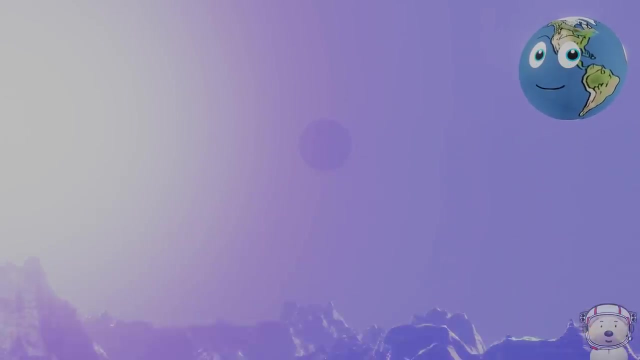 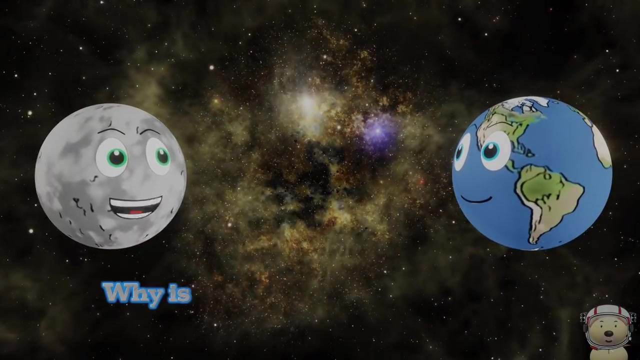 slice. space is silent to humans. think of your favorite space movie and you will see exciting chases with loud spacecraft, cool sounding lasers and massive explosions. yikes, but this is what it would actually sound like to us in space. why is there no sound in space? sound travels in waves and through a water or 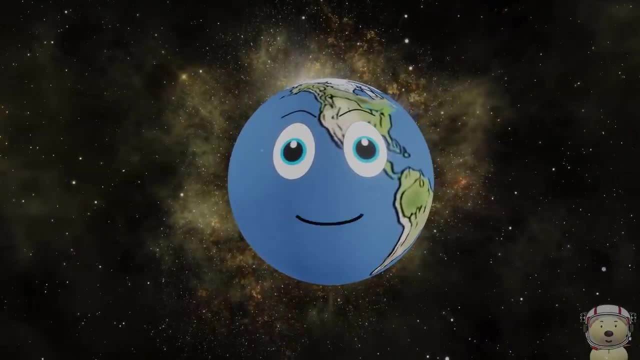 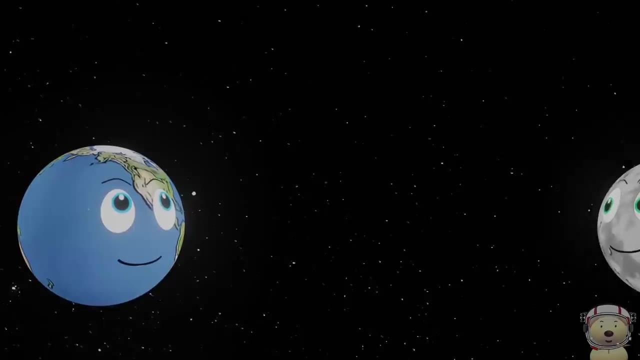 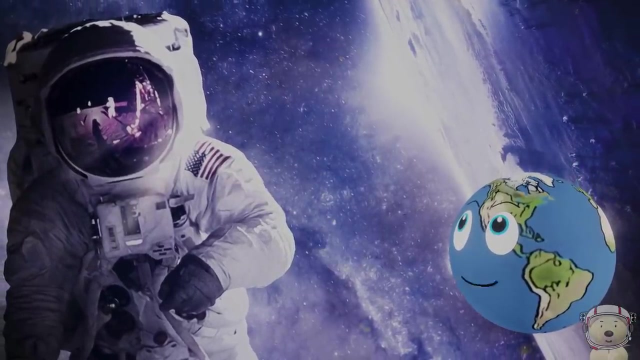 material, but it must have something to travel through. there is no atmosphere in space, which means that the sound has no way to travel. So how do astronauts talk to each other then? They use radios to talk, and on the International Space Station there is an atmosphere, so they 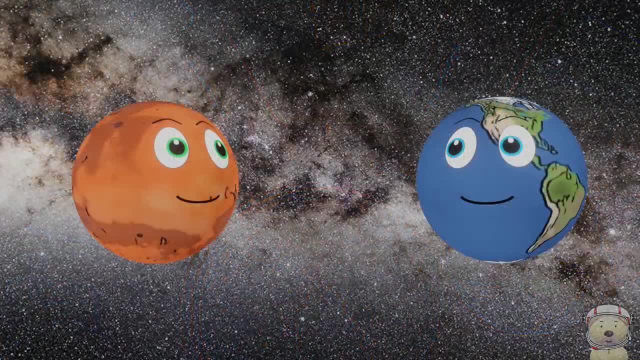 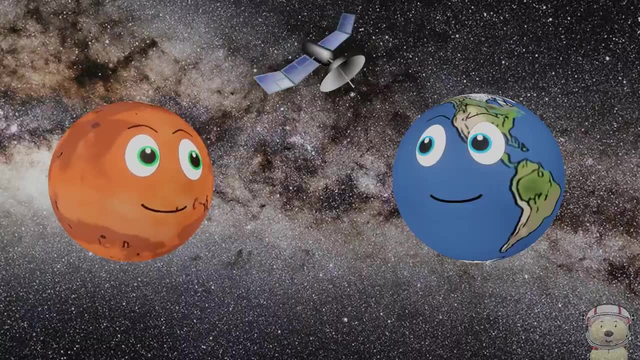 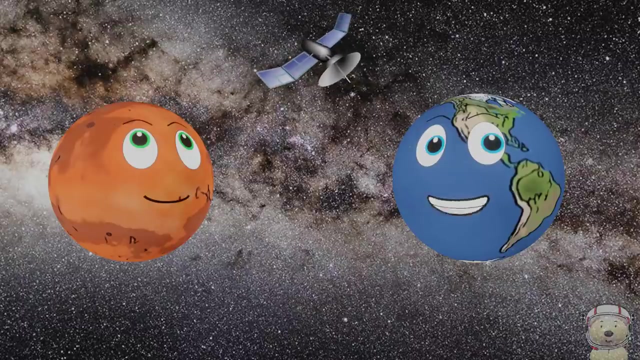 can talk normally. Hey, we can hear the rest of my song now. Satellite, give me a beat. My name is Mars and my sunsets are so cool. Hang on. there's no sound in space. I'm the coolest planet that you know. 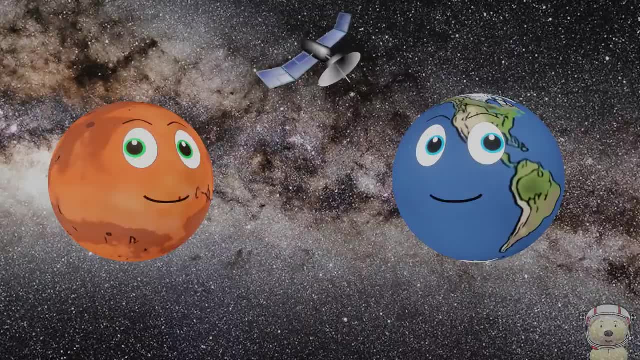 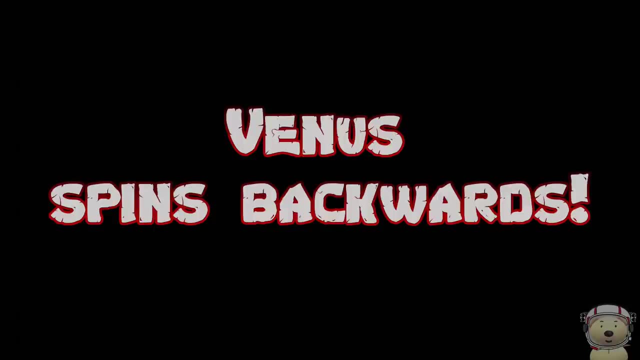 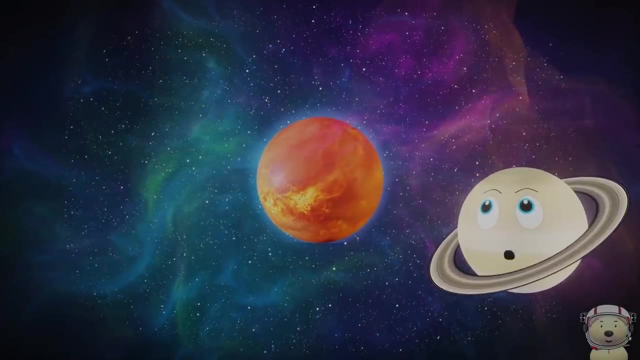 Ah, that's better. Venus spins backwards. Venus is the only planet in the solar system that spins backwards compared to the others. Most planets spin backwards. Venus is the only planet in the solar system that spins backwards compared to the others. Most planets spin backwards. 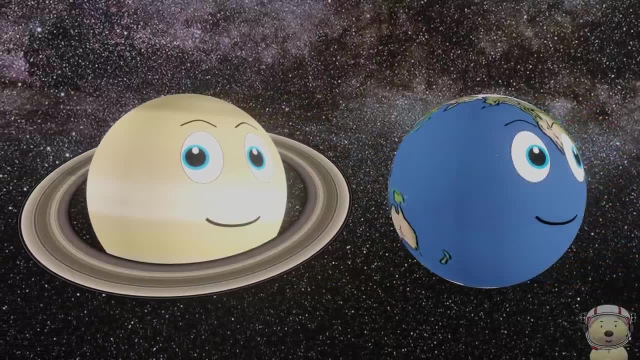 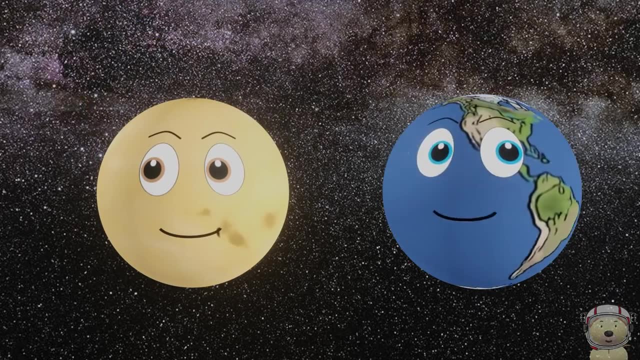 Just like Earth does here. Hey, Earth, Hey. But for some reason Venus spins like this Weird. Go faster, please, just to show them: Faster, Faster, Woah, Woah, Woah, Woah, Woah. 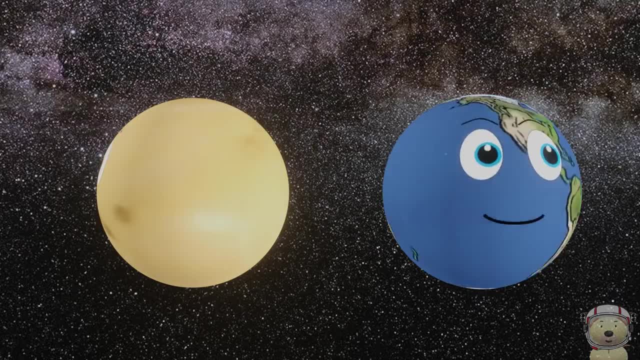 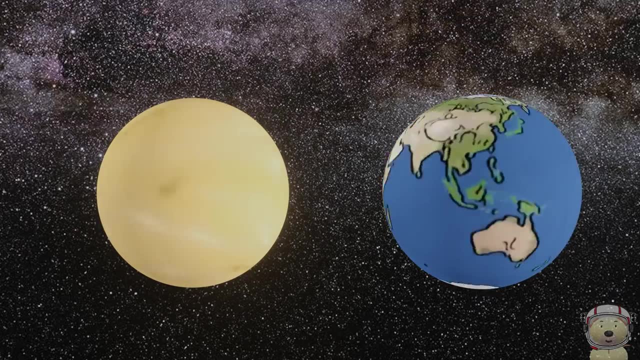